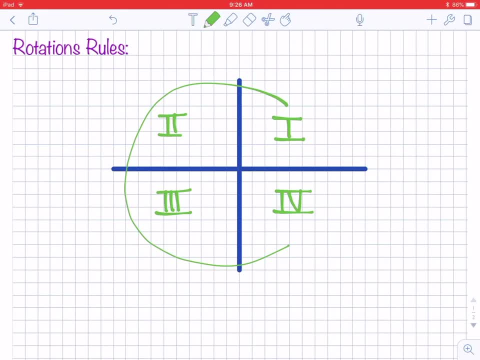 Remember they go in the order of like a letter C. In our first quadrant our signs are always positive, positive. In the second quadrant they are negative, positive. In the third quadrant they are both negative. And in the fourth quadrant the signs are positive, negative. 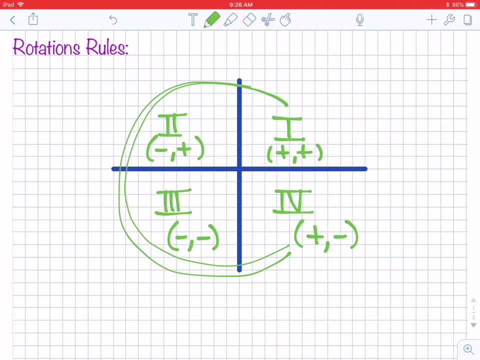 So remember, it's like the letter C would be written and that's the order they go in. Now let's add in a way to remember our rotation rules that kind of coordinates with these quadrants. So in our first quadrant we're just going to put our basic points X and Y. 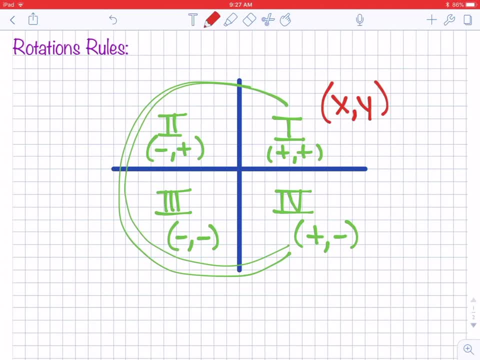 And in the third quadrant, which is 180 degrees away, we're going to put negative X And negative Y, And then in the second and the fourth quadrant we need to switch the X and the Y. So I'm going to write that down and then add in your signs. 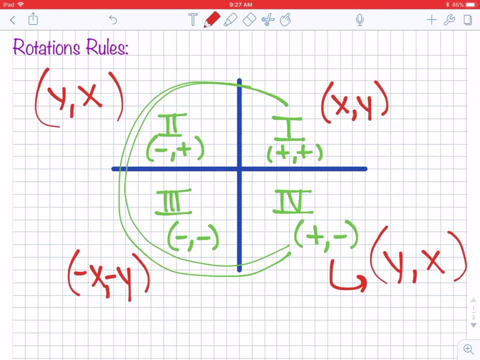 So just like the fourth quadrant would always be positive, negative, And just like the second quadrant would always be negative, positive. Now we have all of our rotation rules that we can easily pick from. So let's say that we are told that a figure is rotated 90 degrees. 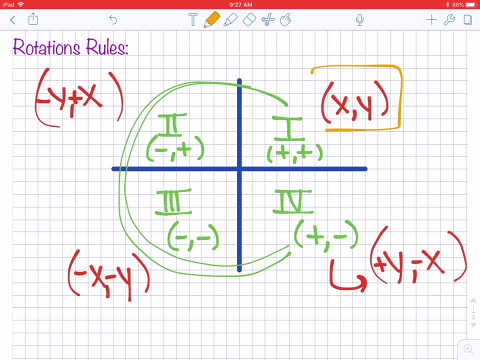 90 degrees clockwise, Then I would just start here and go 90 degrees clockwise, And then that would be what I need to do with my points to figure out what the image would be. So let's try another one, Like, let's say that the figure we're given, say a triangle ABC is going to be rotated 270 degrees counterclockwise. 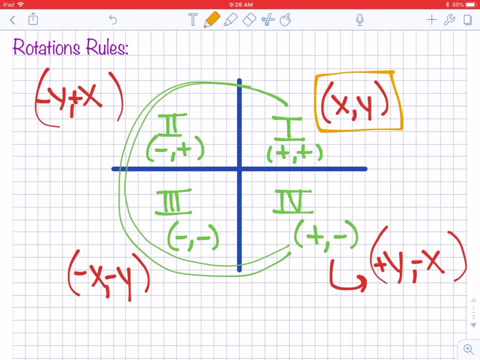 So again, start with your basic pair of points, X, Y, But go three quadrants counterclockwise, And that is your rule, So you'd be able to figure out what the points for the image would be, or your range. 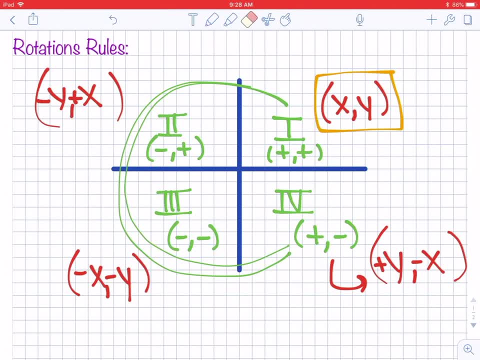 All right, let's try another one. So let's say I want to rotate a figure 180 degrees. Remember, it doesn't matter if you go counterclockwise or clockwise, That rule stays the same. So, starting from X and Y, you would end up with negative X, negative Y.